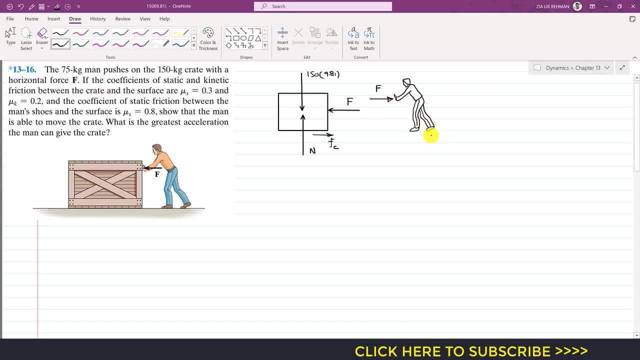 And then if the force is applied on the main in this direction. So what will happen is that there will be a friction force between the shoes and the surface Right, And let's say that this is the friction for main Right. So now, if I consider this crate as a free body diagram, 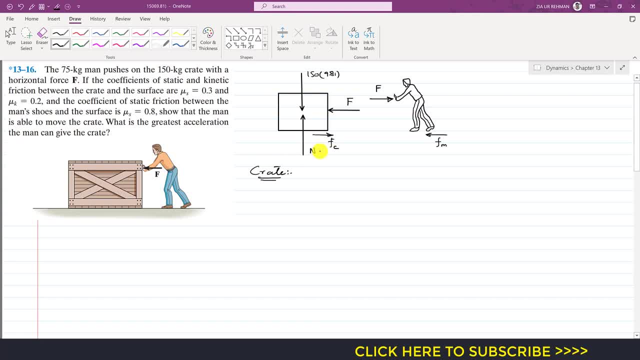 And if I apply the equilibrium conditions Right, Since we want to move this 150 kg crate Right. So in order to move this 150 kg crate, This friction force need to be equal to that maximum friction Right That is offered by the surface to this crate. 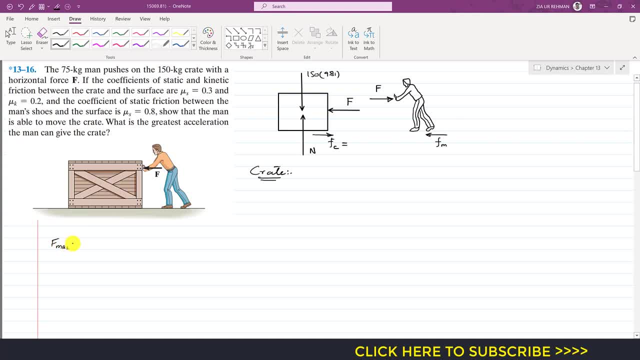 Right. So the maximum friction Between the crate and the surface Is will be equal to mu s time n Right, And, if we apply the summation of forces along y, equals to 0.. Since, just before starting the motion, the system is in equilibrium. 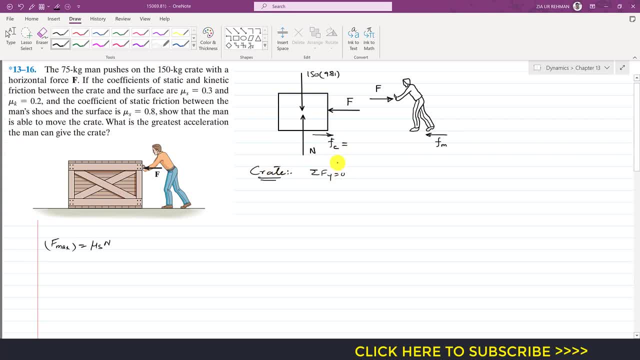 Right, So we are considering the equilibrium conditions, Right? So if we apply, the summation of forces along y equals to 0.. So that will mean that the n minus weight, This will be equal to 0.. Or we can say that the normal force is equal to the weight. 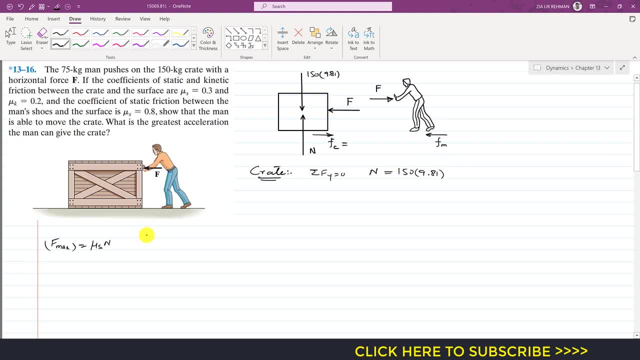 Of the crate Right. So from this we can say that the maximum friction That the surface can offer to the crate will be equal to mu s, and mu s is 0.3.. So I will write 0.3 times that n, which is 150 x 9.81.. 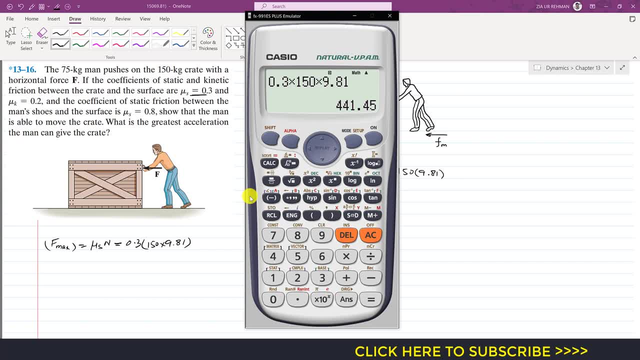 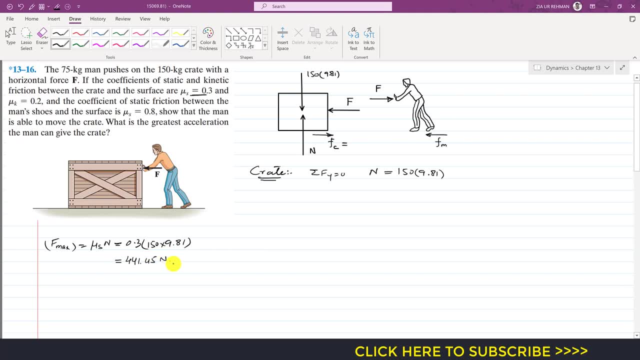 So this is equal to 441.45.. So I will write that this is 441.45.. Right, 41.45 newtons, right. so now we want to move this crate. so, just before moving the crate, this friction force will be maximum and that friction force will be equal to this maximum friction. 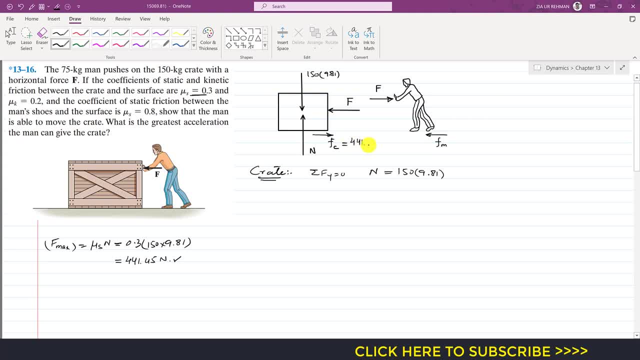 right. so we can write that this fc is known for the particular case, which is 441.45 newtons. so now, if i apply the summation of forces along, x equals to zero. if this is my positive x direction, this is my positive y direction. so, as we can see that this friction force is acting in the negative, 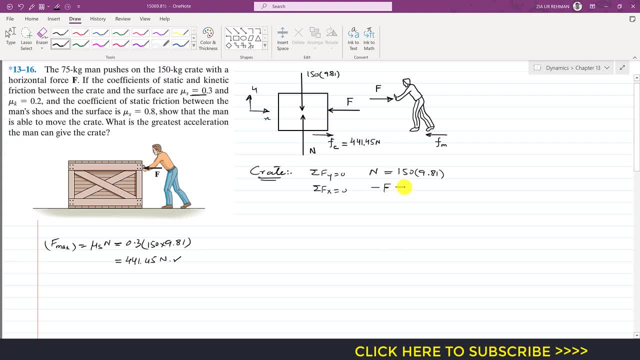 x direction. so i have tried: minus f and this will be plus this fc, which is equal to that maximum friction. so this is 441.45 and this is equal to zero, or we can say that f is equal to 441.45 newtons. right, so now in order to move. 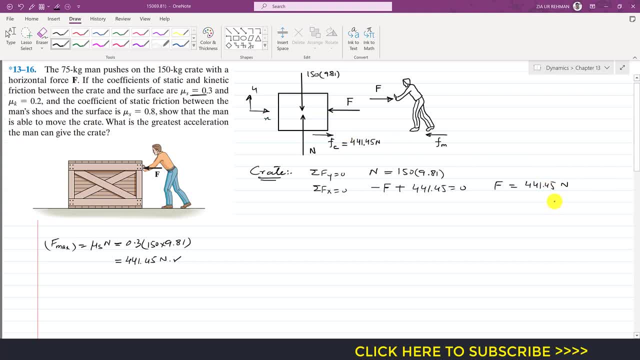 this y 150 kg create the main needs to apply at least 441 point four five Newton force in order to overcome that friction, that maximum friction that surface can offer Right. so the moment can be initiated when the force is greater than equal to the external applied force by the main is greater. 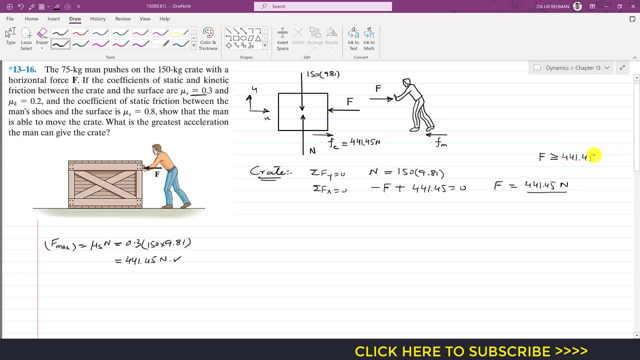 than equal to 441 point four five Newton. The force less than this particular value will not initiate any motion, will not move the the crate Right. So now this means that if we consider this as the free body diagram, then this F is At least need to be equal to four hundred and forty one point four five Newton right. 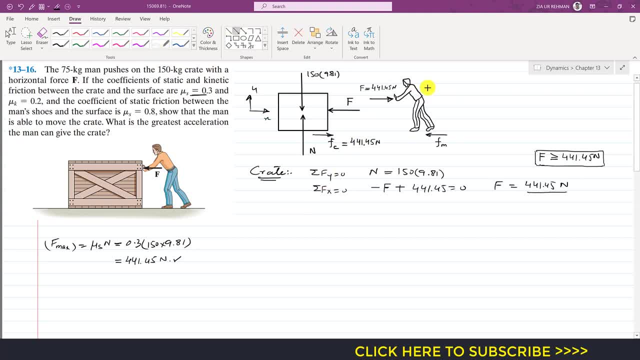 so now again the, The man has its own weight which will be acting vertically downward, and that Weight is seventy five times Nine, point eight, one and again the surface will apply the normal force Right, So I am considering this resultant normal force on main right. So now again, if we apply the, 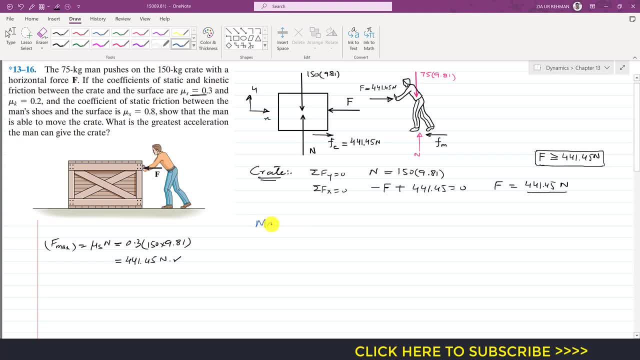 Equilibrium condition to the body of man, right. So let me write that we are considering now the main. So now, if I apply the summation of forces along y equals to zero. right again, we are Considering the equilibrium conditions, right. So now, from this we can say that this N is acting in the positive y direction. 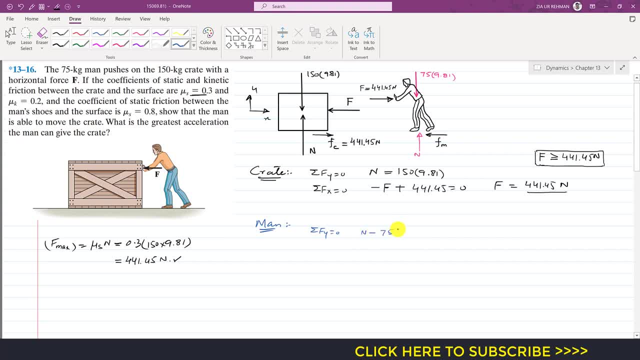 So I have to write plus n, minus that weight of the main, which is 75, into nine point eight one, and This is equal to zero. or we can say that n is equal to the weight of the main right. similarly, if I apply the summation of forces along, x equals to zero. then, as we can see that this F is acting in the 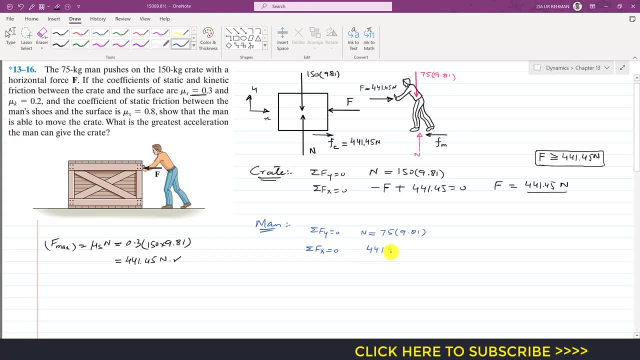 positive x direction. so I have to write four hundred and four: 441.45 minus the friction for main will be equal to zero. or we can say that the friction that will occur between the shoes and the surface when this much force is applied on the crate will. 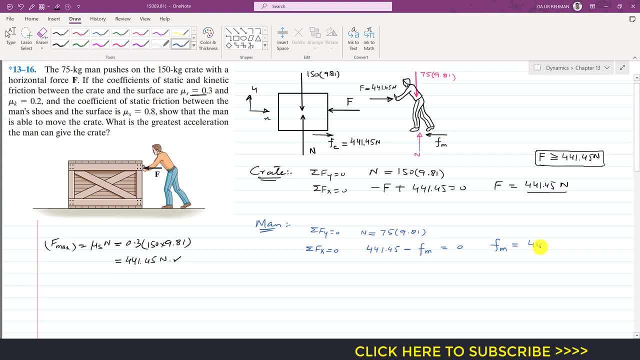 be equal to 441.45 newtons right and the maximum friction that the surface can offer to the shoes of the main will be equal to. so let me write: this is the maximum friction for crate right. so this is the maximum friction for main and this will be equal to mu s and again for main, mu s is. 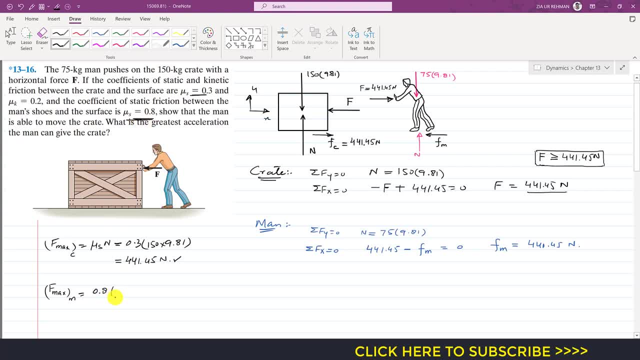 0.8. right, so now i will write 0.8. so now i will write 0.8. so now i will write 0.8. times n and for main is the weight of the crate. times n and for main is the weight of the crate. 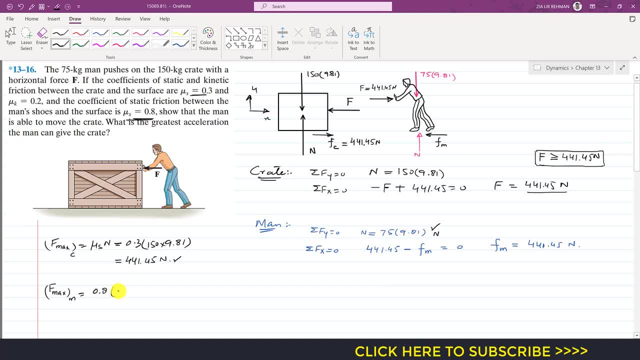 times n, and for main is the weight of the crate now, the weight of its uh of its body right now. the weight of its uh of its body right now. the weight of its uh of its body right so now this will be 75 times. so now, this will be 75 times. 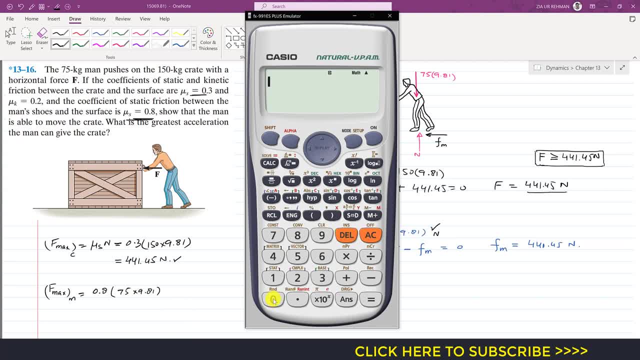 so now this will be 75 times 9.81. so this is 0.8 times 75 times 9.81. so this is 0.8 times 75 times 9.81. so this is 0.8 times 75 times 9.81, and this gives me 588.6. 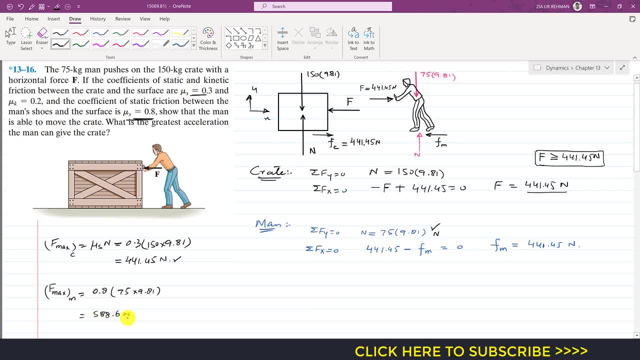 9.81, and this gives me 588.6, 9.81, and this gives me 588.6, so 588.6, so 588.6, so 588.6. newtons right so now. newtons, right so now. newtons, right so now. when the man applies at least this much. 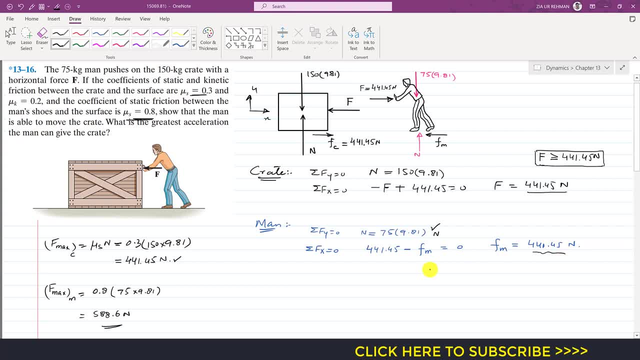 when the man applies at least this much, when the man applies at least this much force, so this much friction is developed force, so this much friction is developed force, so this much friction is developed, and this friction is less than that, and this friction is less than that. 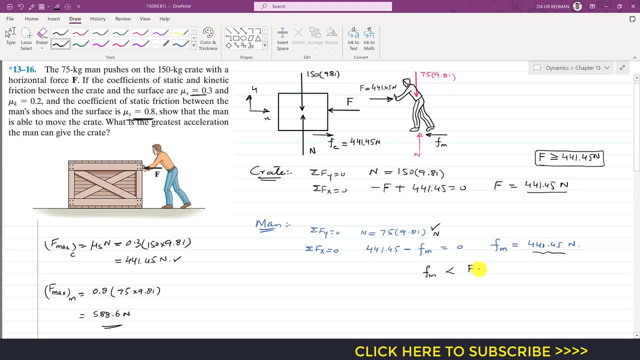 and this friction is less than that maximum friction that the surface can, maximum friction that the surface can, maximum friction that the surface can offer to the shoes of the man, offer to the shoes of the man, offer to the shoes of the man, right so f max man. 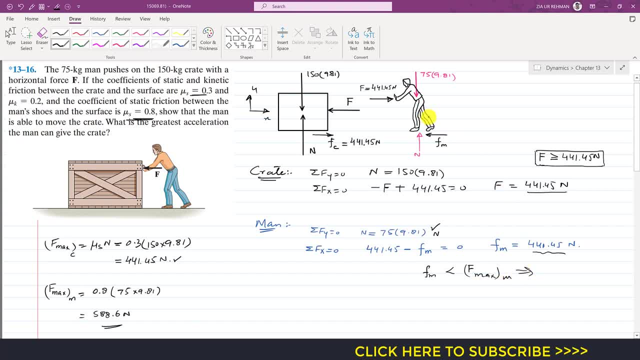 right, so f max man. right, so f max man. so from this we can conclude that. so from this we can conclude that. so from this we can conclude that the man is not going to slip right. so if the man is not going to slip right, so if 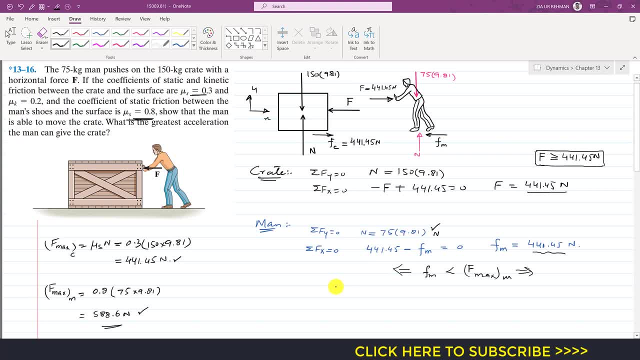 the man is not going to slip right. so if the man is not slipping so he is able to, the man is not slipping so he is able to. the man is not slipping so he is able to move this crate, move this crate, move this crate. in the problem statement is said that show 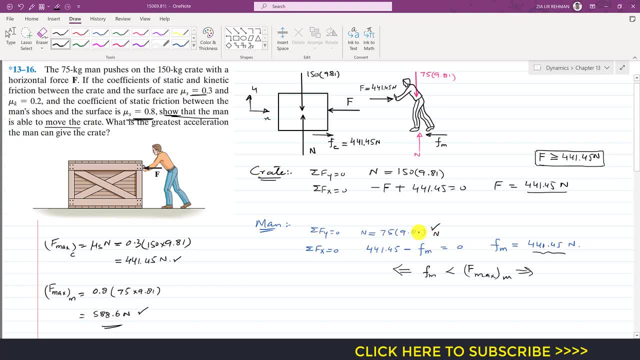 in the problem statement is said that show in the problem statement is said that show that the man is able to move the crate, that the man is able to move the crate, that the man is able to move the crate. yes, the man is able to move the crate. 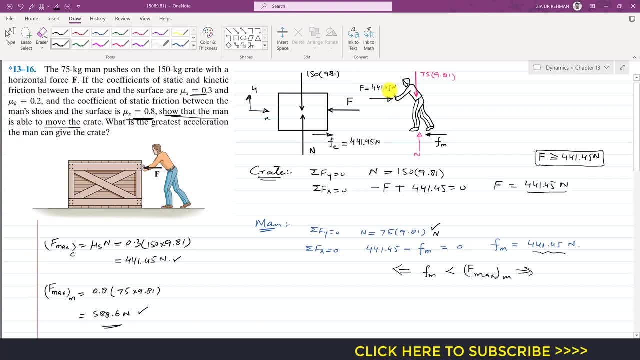 yes, the man is able to move the crate. yes, the man is able to move the crate, since if he applies uh 441.45 newton, since, if he applies uh 441.45 newton, since, if he applies uh 441.45 newton force, so he will not slip. 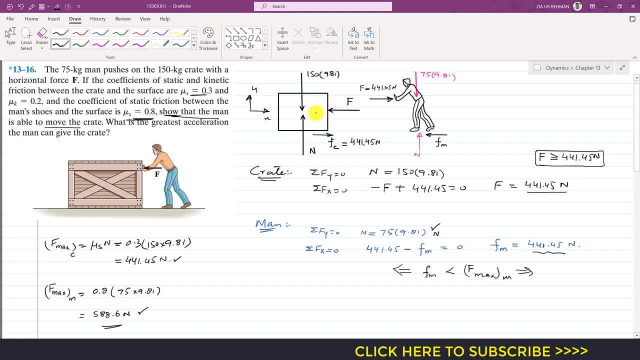 force, so he will not slip. force, so he will not slip. and in the other case, and in the other case, and in the other case, the crate will move right, the crate will move right, the crate will move right, but he will not slip until and unless. but he will not slip until and unless. 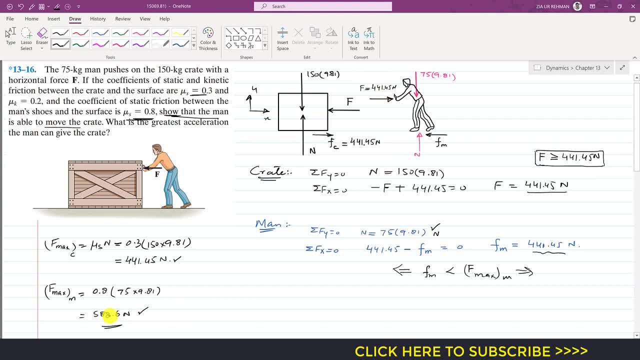 but he will not slip until and unless this external force f, this external force f, this external force f is greater than or equal to this 588.6 is greater than or equal to this 588.6 is greater than or equal to this 588.6. right, so he, the main need to push the 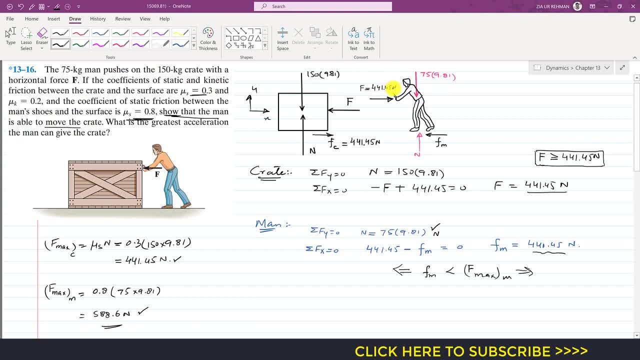 right. so he the main need to push the right, so he the main need to push the crate with crate, with crate, with four at least 441.45 newtons right, four, at least 441.45 newtons right, four at least 441.45 newtons right. and in the problem statement now it is: 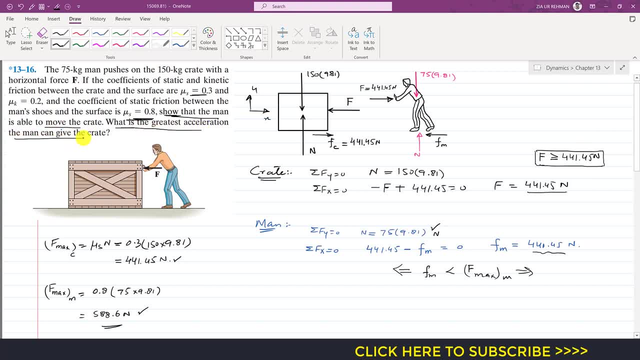 and in the problem statement now it is. and in the problem statement now it is, said that what is the greatest. said that what is the greatest, said that what is the greatest acceleration the man can give to the acceleration the man can give to the acceleration the man can give to the crate. 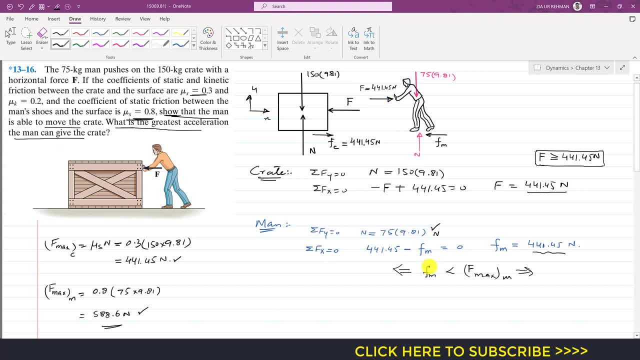 crate, crate, right, so the man can apply a maximum right, so the man can apply a maximum right, so the man can apply a maximum force of force, of force of how much the maximum force of this much, how much the maximum force of this much, how much the maximum force of this much right. 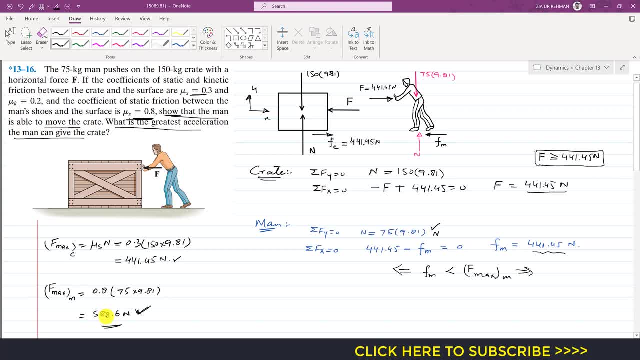 right, right. he cannot increase the force. he cannot increase the force. he cannot increase the force, then 588.6 newton, otherwise he will then 588.6 newton, otherwise he will then 588.6 newton, otherwise he will slip right. so in order to have 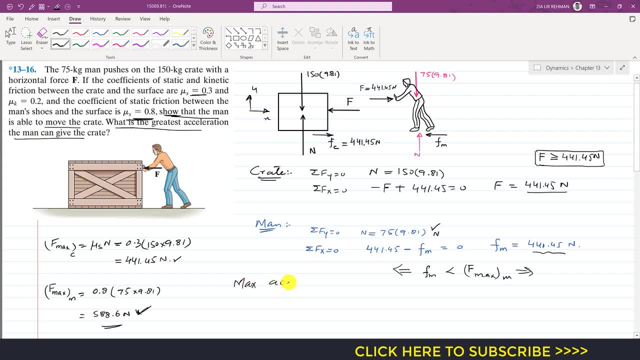 slip right. so, in order to have slip right, so in order to have maximum, maximum, maximum acceleration, acceleration, acceleration, the force, the external force, the force, the external force, the force, the external force, need to be equal to or less than, need to be equal to or less than. 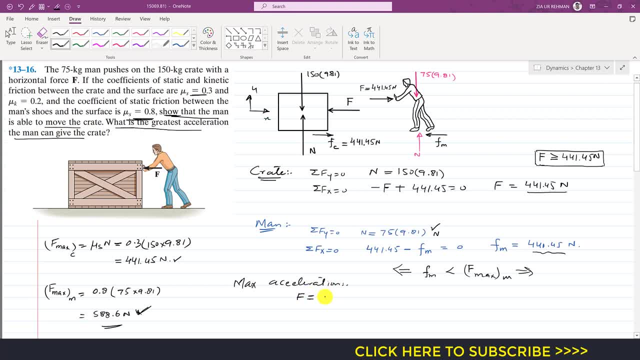 need to be equal to or less than if, if we want to have maximum solution, if, if we want to have maximum solution, if, if we want to have maximum solution, so then that external force need to be, so, then that external force need to be, so then that external force need to be equal to that f. 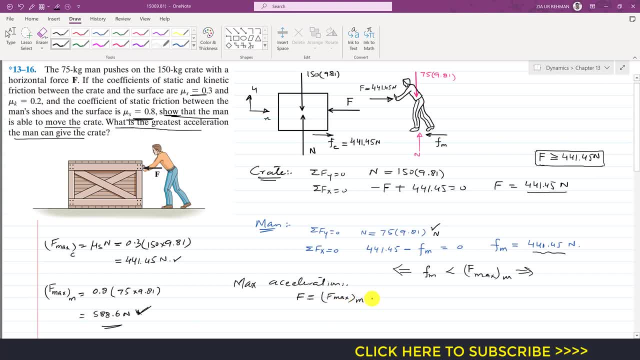 equal to that f, equal to that f max for man. max for man. max for man, right just before slipping. so this will right just before slipping, so this will right just before slipping. so this will be 588.6 be, 588.6, be, 588.6 newtons. right, so now. 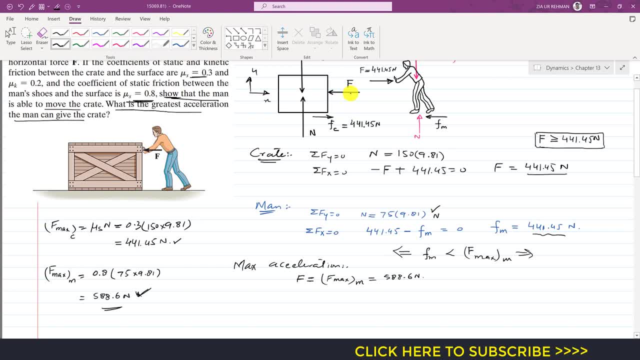 newtons right, so now. newtons, right, so now. if this is the case, if the force is, if this is the case, if the force is, if this is the case, if the force is equal to, equal to, equal to 588.6 and this force is greater than. 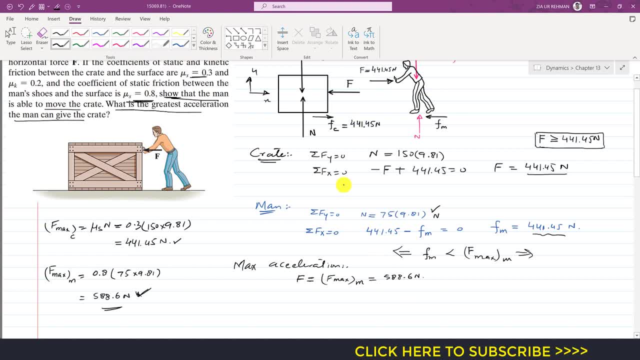 588.6, and this force is greater than 588.6, and this force is greater than 441.45. so what will happen is that this 441.45. so what will happen is that this 441.45. so what will happen is that this force will overcome this friction force. 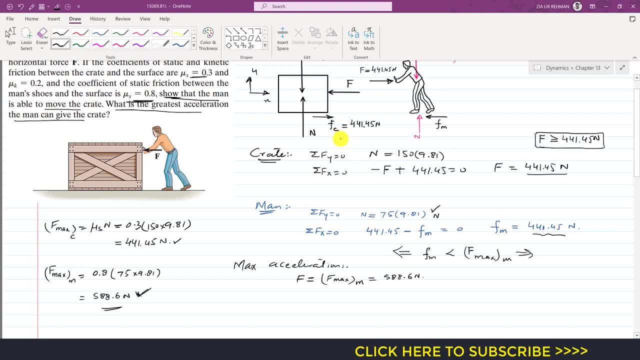 force will overcome this friction force. force will overcome this friction force, and it will, and it will, and it will, uh, it will move the crate. it will, uh, it will move the crate. it will, uh, it will move the crate. it will accelerate the crate right. accelerate the crate right. 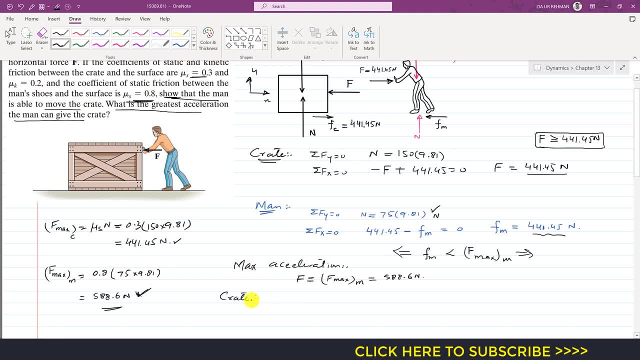 accelerate the crate right. so now if we apply again, if i consider so, now if we apply again, if i consider so, now if we apply again, if i consider the crate, and now if i apply the the crate, and now if i apply the the crate, and now if i apply the equation of motions in the x direction. 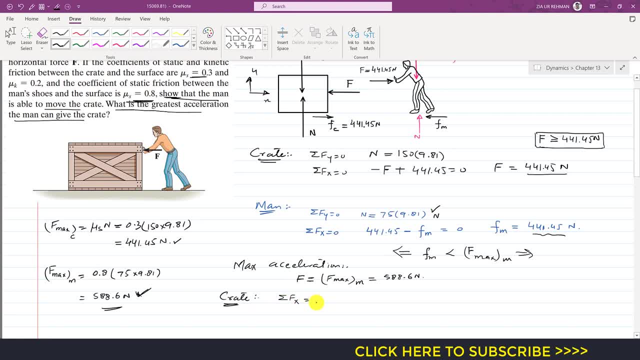 equation of motions in the x direction. equation of motions in the x direction. now, if i apply now, if i apply now, if i apply, the summation of force along x equals to the summation of force along x. equals to the summation of force along x. equals to m, a, x, right. 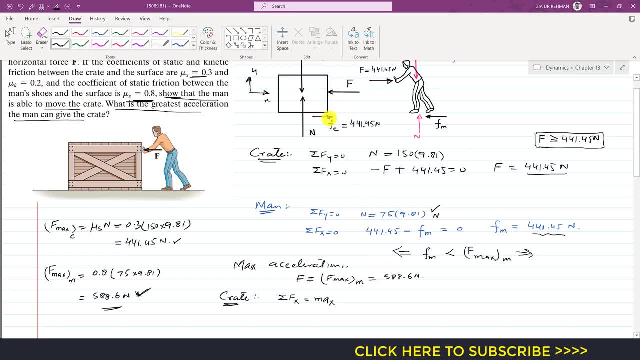 m a x right, m a x right. so now as we can see that, uh, so now as we can see that, uh, so now as we can see that, uh, this friction force is acting in the. this friction force is acting in the. this friction force is acting in the negative x direction. so i will write. 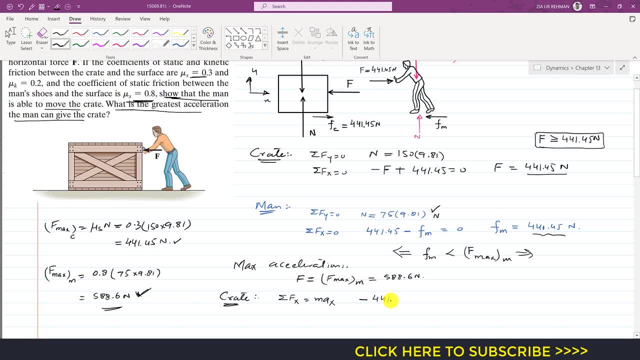 negative x direction. so i will write negative x direction, so i will write minus, and that is 441 minus, and that is 441 minus and that is 441 now, since the crate will be moving, then now, since the crate will be moving, then now, since the crate will be moving, then the friction force will not be. 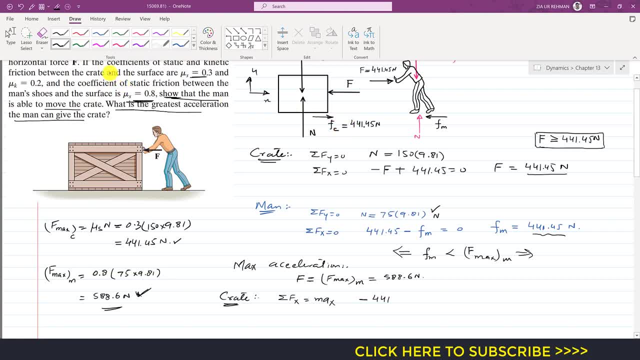 the friction force will not be. the friction force will not be this friction, it will be that friction, this friction, it will be that friction, this friction, it will be that friction due. uh, that will be kinetic friction due. uh, that will be kinetic friction due. uh, that will be kinetic friction. right, so now. 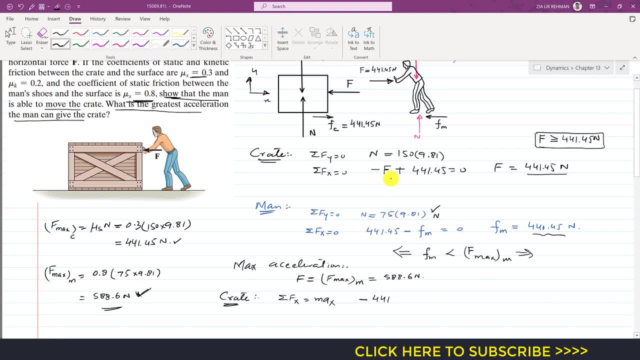 right, so now. right, so now. we need to write to apply the equation. we need to write to apply the equation. we need to write to apply the equation of motion. we need to consider the of motion. we need to consider the of motion. we need to consider the kinetic friction here. right, so let me. 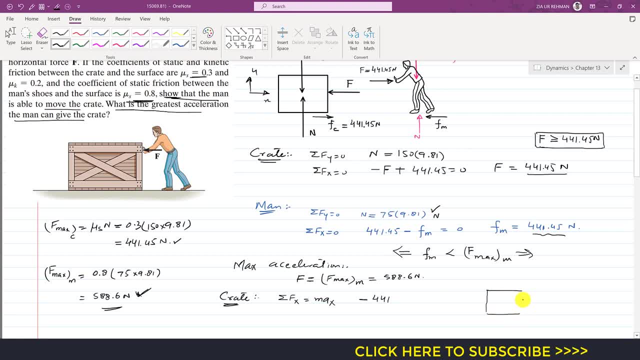 kinetic friction here, right so let me. kinetic friction here, right so let me draw the free body diagram when it is. draw the free body diagram when it is. draw the free body diagram when it is moving, moving, moving when the crate is moving- right, so now in the crate is moving, then this will be the weight, this will be the normal force. 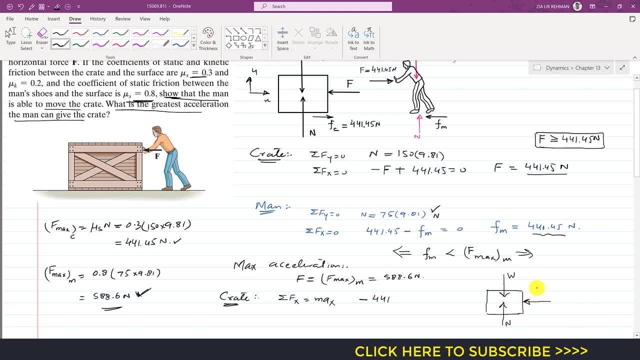 and now the. the external applied force is equal to 588.6 newton and the friction force will be equal to mu k times n, right? so now we can write that and this will be mu k times n. so i will write minus n. mu k for the crate is 0.2, right, so i have to write 0.2 times n, and n is equal to the weight. 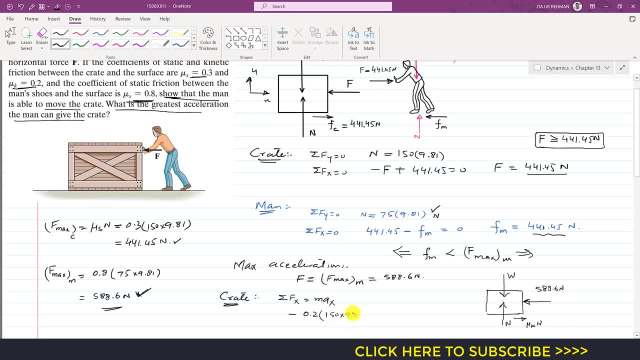 of the crate, which is 150 times 9.81, minus that f, which is 588. uh, this is acting in the positive direction, right? this is our positive direction and this is our positive y direction, right? so this is acting in the positive x direction. this is acting in the negative x.